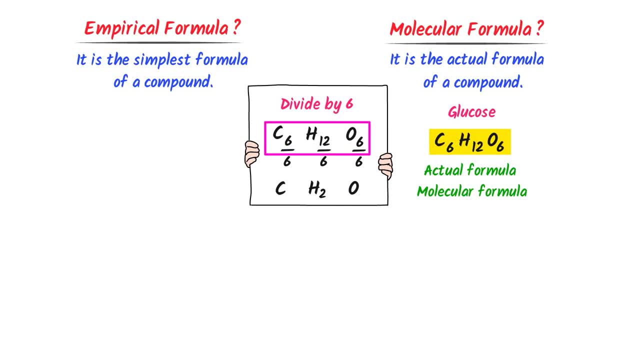 a glucose from C6H12O6 to CH2O6.. Now listen carefully. I have simplified the molecular formula of a glucose from C6H12O6 to CH2O6.. This CH2O is the simplest formula of a glucose. 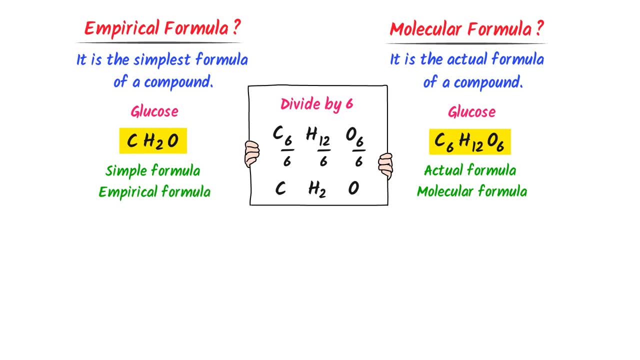 Hence it is the empirical formula of a glucose. Thus we learn that molecular formula is the actual formula of a compound like C6H12O6, while empirical formula is the simplest formula of a compound like CH2O. Remember that molecular formula is equal to n times of empirical formula. 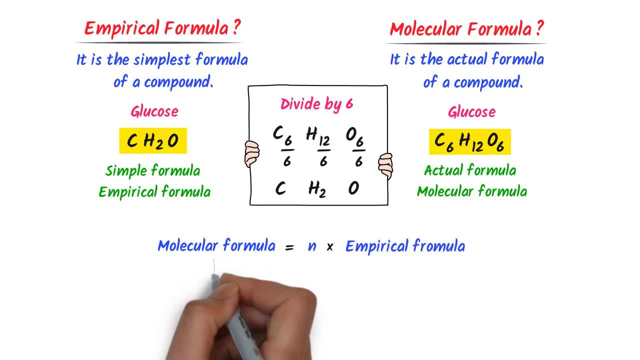 For example, the molecular formula of a glucose is C6H12O6, while its empirical formula is CH2O. Here the value of n is 6.. I mean, if we multiply the subscripts of empirical formula by 6, we will get molecular formula. Therefore we say that molecular formula is equal to. 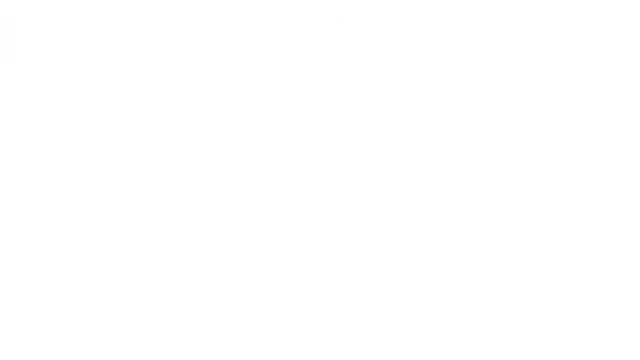 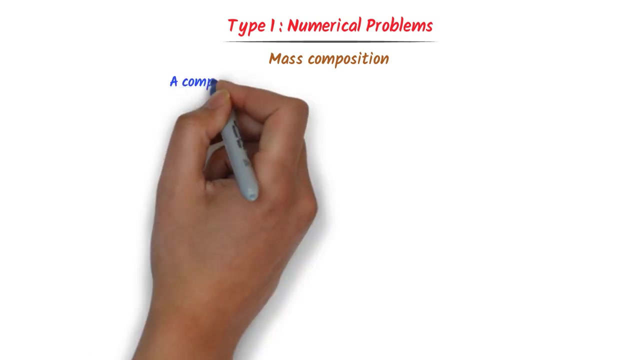 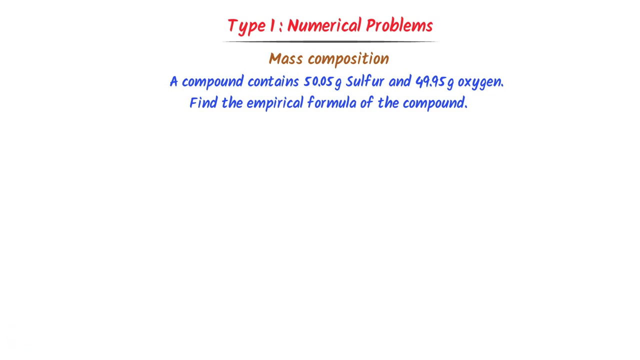 n times of empirical formula. Now let me teach you Type 1 Form Numericals, which we call mass composition. Consider this problem: A compound contains 50.05 g sulfur and 49.95 g oxygen. Find the empirical formula of this compound. Well, in such type of numerical problems, we are given masses of the different. 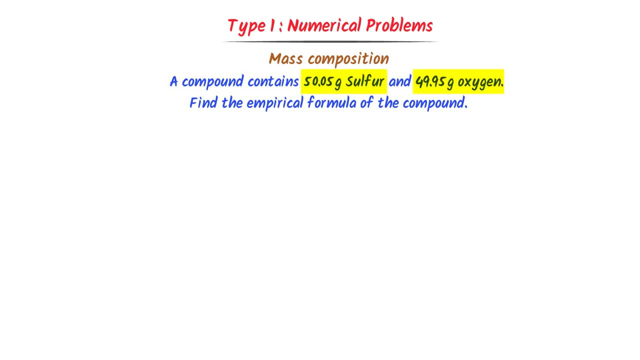 atoms like 50.05 g of sulfur and 49.95 g of oxygen. In this type of numerical problem we get factor number of О, which is equal to the weight of the right-hand side of the change, and number of the left-hand side, of the right-hand side of the change and the 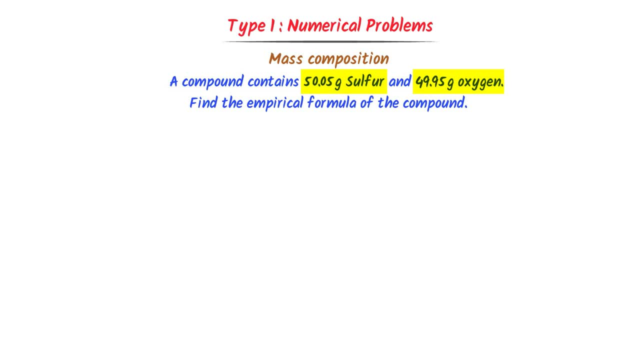 0.95 gram of oxygen and we are asked to find the empirical formula of a compound. I solve such type of numerical problems with the help of three steps. In the first step, I write the given atoms, which are sulfur and oxygen. 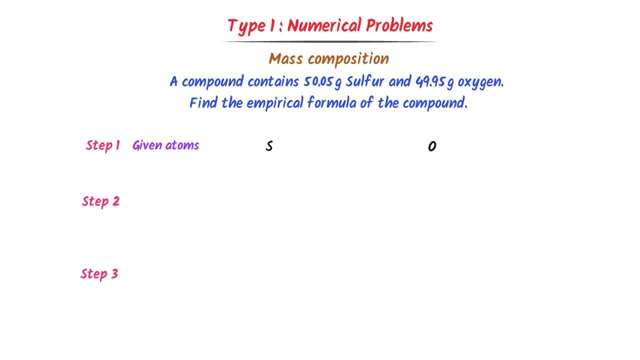 Secondly, I write their respective gram atomic masses. For example, the gram atomic mass of sulfur is 32 gram and that of oxygen is 16 gram. In the second step I calculate the number of moles of given masses. For example, the given mass of sulfur is 50.05 gram and the given mass of oxygen is 49.95. 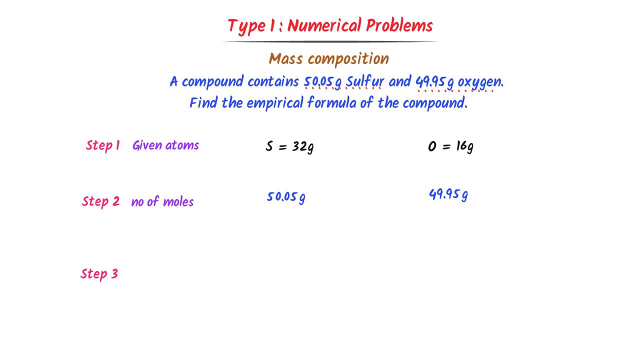 gram. Now to find the number of moles, I divide the given mass by their respective atomic masses. The gram atomic mass of sulfur is 32 gram. I divide the given mass by 32.. The gram atomic mass of oxygen is 16 gram. 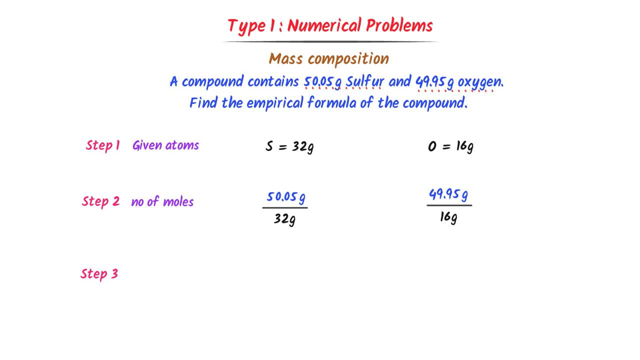 I divide the given mass by 16.. After calculation, I get 1.56 moles of sulfur and 3.12 moles of oxygen. In the third step, I find the simplest ratio between atoms. To do so, I rewrite the number of moles of each atom. 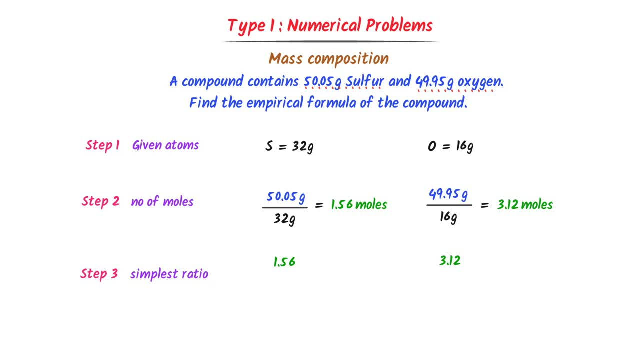 Now I select the smallest number. We can see that 1.56 is the smallest number. I select this number. I divide 1.56 by 1.56 and 3.12 by 1.56.. After calculation I get 1 and 2.. 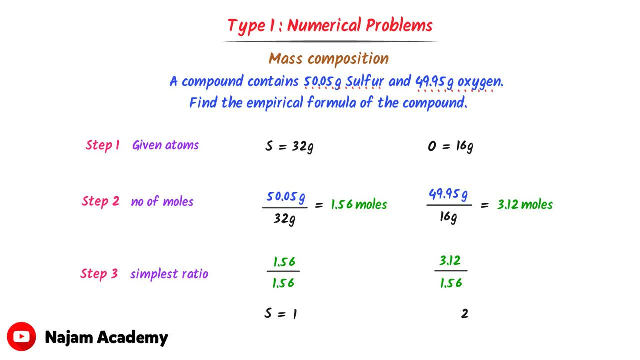 It means that the ratio of sulfur is 1 and that of oxygen is 2, and the compound. Thus I write S1O2.. This is the empirical formula of this compound. Therefore, using these three steps, we can easily calculate the ratio of sulfur to oxygen. 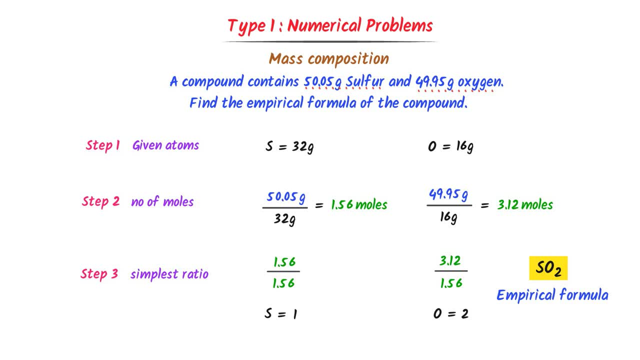 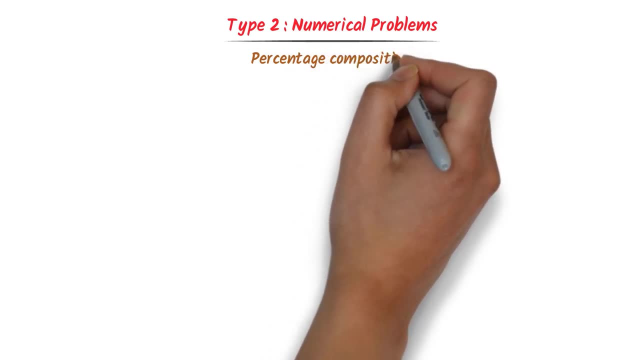 We can easily calculate the ratio of sulfur to oxygen. We can easily calculate the ratio of sulfur to oxygen. We can easily calculate the empirical formula of any compound. Now let me teach you the second type of numerical problems, which we call percentage composition. 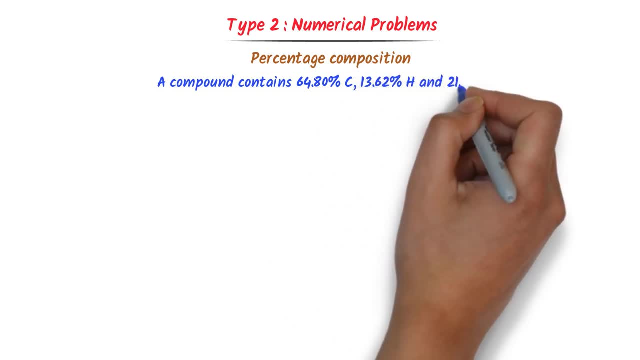 Consider this numerical problem. A compound contains 64.8% carbon, 13.62% hydrogen and 21.58% oxygen-by-weight. Find the empirical formula of this compound. Well, in this type of numerical problems, percentage composition is calculated as following: 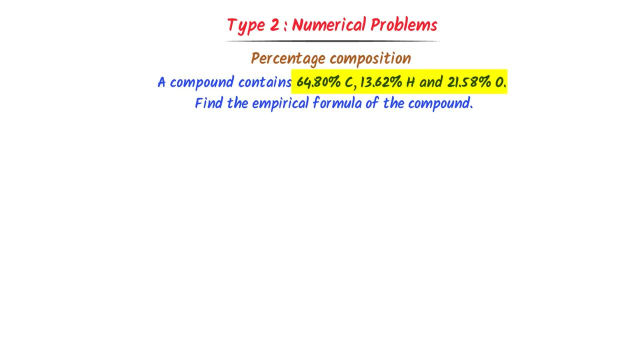 In this type of numerical problems, percentage of different atoms are given, But we consider them as masses of atoms in grams. I mean, instead of percentage, I consider them in grams like 64.8 g of carbon, 13.62 g of 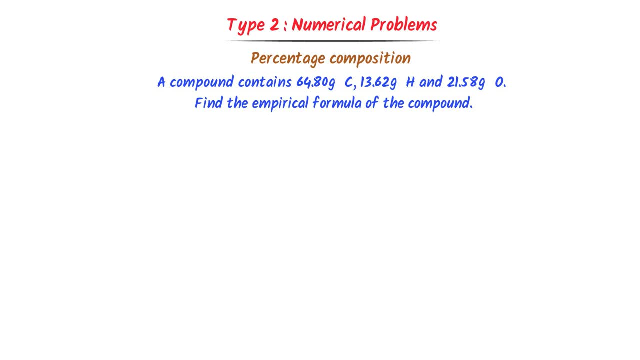 hydrogen and 21.58 g of oxygen. So this numerical has become like first type of numerical problem. Hence I will solve it using the previous three steps, which we already learned. In the first step I write the given atoms, like carbon, hydrogen and oxygen. 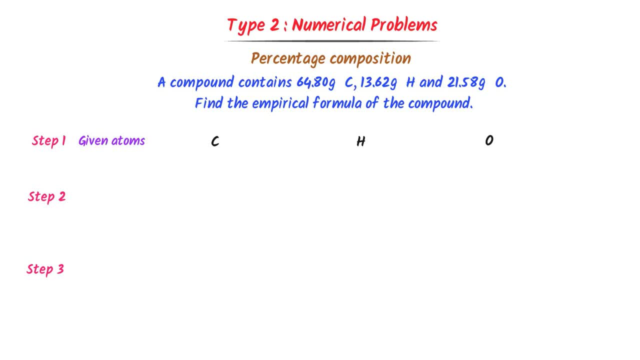 Secondly, I write their respective atomic masses. The atomic mass of carbon is 12 g, that of hydrogen is 1 g and that of oxygen is 16 g. In the second step I find the number of moles of given masses. 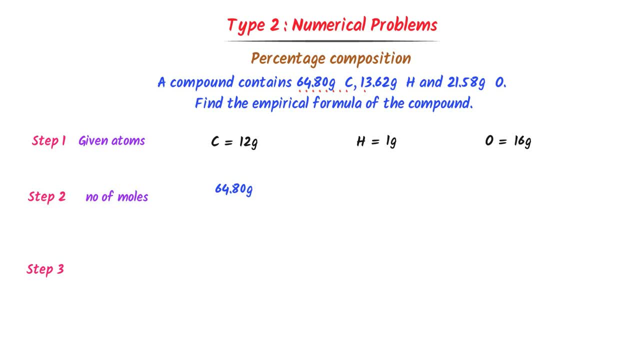 The given mass of carbon is 16 g. The given mass of carbon is 16 g, The given mass of hydrogen is 13.62 g and the given mass of oxygen is 21.58 g. I divide these given masses by respective atomic masses, like 12 g of carbon, 1 g of 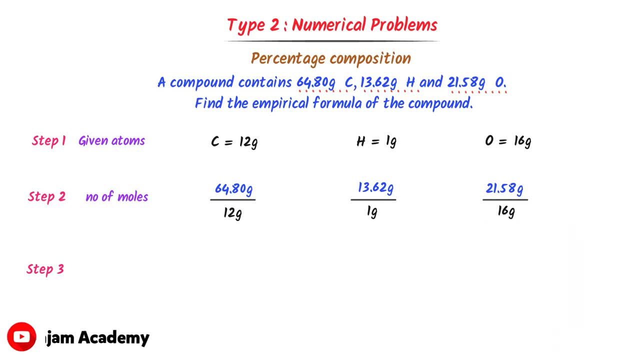 hydrogen and 16 g of oxygen. After calculation I get 5.4 moles of carbon, 13.62 moles of hydrogen and 1.35 moles of oxygen. In the third step I find the simplest ratio between atoms. 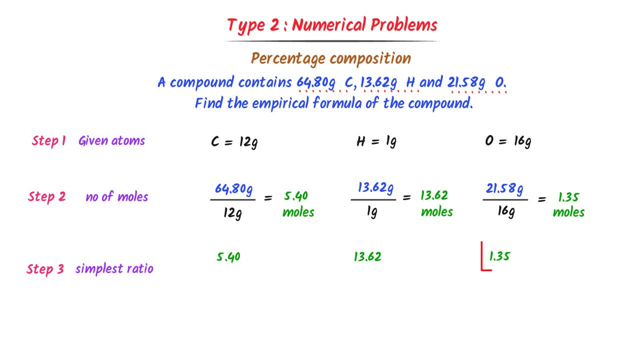 I rewrite the number of moles. Now the smallest number is 1.35.. I select it and divide all these numbers by 8.. 5.4 by 1.35, 13.62 by 1.35 and 1.35 by 1.35.. 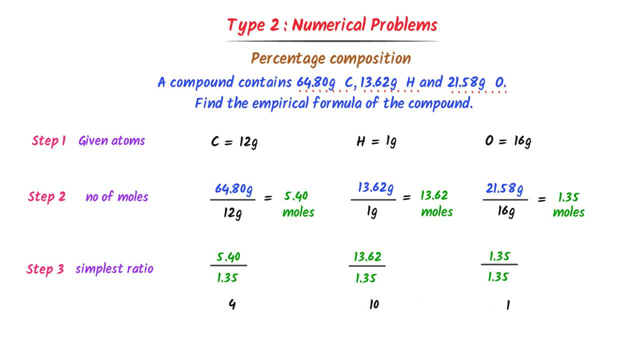 After calculation I get 4,, 10 and 1.. Now I write the number of moles of oxygen. In the third step I find the simplest ratio between atoms. It shows that the ratio of carbon is 4,, that of hydrogen is 10, and that of chlorine is. 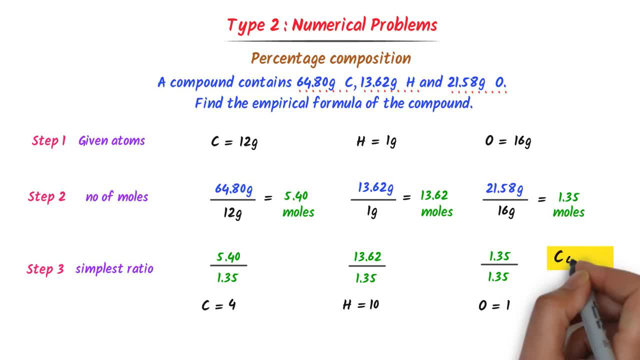 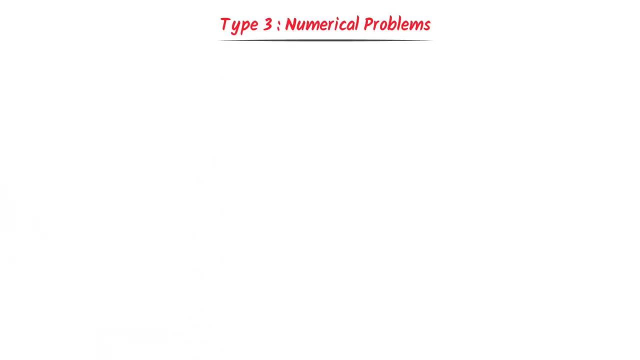 1.. Hence, the empirical formula of the compound is C4H10O1.. Therefore, using these three steps, we can easily find the empirical formula of any compound. Now let me teach you Type-III forms of numerical problems, which we call calculating molecular. 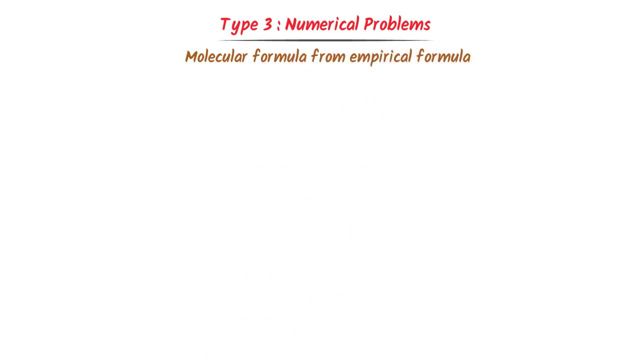 formula from empirical formula formula, For example, consider this problem: Calculate the molecular formula of a compound with the empirical formula BH3 and its molar mass is 27.7 g. Well, in such type of numerical problems, empirical formula is given like BH3.. Secondly, molar mass of the empirical 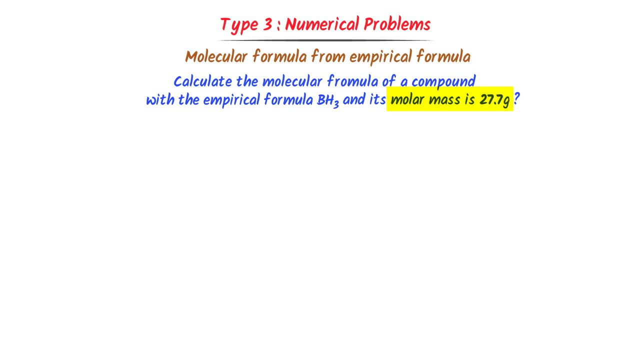 formula is given like 27.7 g. I solve such type of numerical problems using two steps. In the first step I find the molar mass of empirical formula. We know that the given empirical formula is BH3.. I find its molar mass, I write B plus three H, The g atomic. 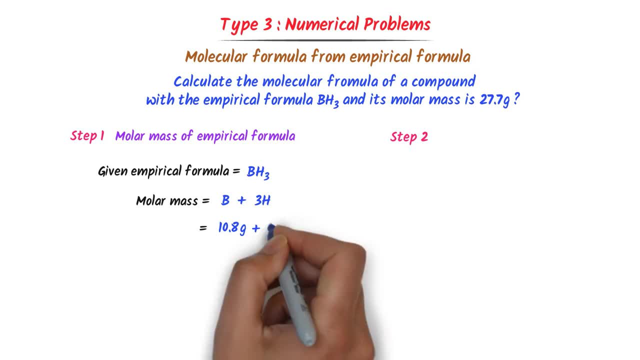 mass of boron is 10.81 g And that of hydrogen is 1 g, 1 g. After addition I get 13.81 g. So the empirical mass of BH3 is 13.81 g. In the second step I find the value of N. To find its value I divide, given mass of. 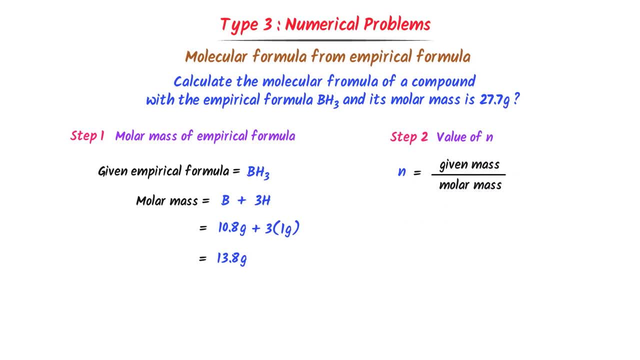 empirical formula. by molar mass of empirical formula, The given mass is 27.7 g and the empirical formula mass is 13.81 g. After division I get N is equal to 2.. We already learned that molecular formula is equal to N times empirical formula. Also, we know that 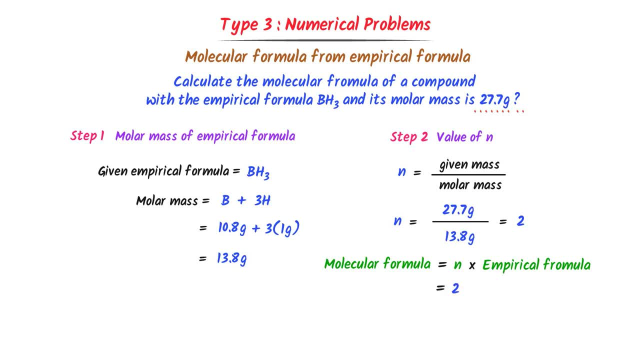 the value of N is 2.. The empirical formula is already given, which is BH3.. I multiply the subscript of empirical formula by 2. I get B2H6.. Hence the molecular formula of this compound is B2H6. Hence, note it down. 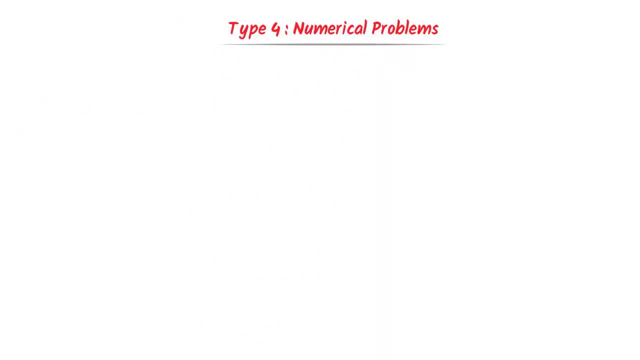 Lastly, let me teach you the four types of numerical problems, which we call calculating, empirical formula and molecular formula. For example, consider this problem: A compound contains 24.27 percent carbon, 4.07 percent hydrogen and 71.8 percent phosphorus. For 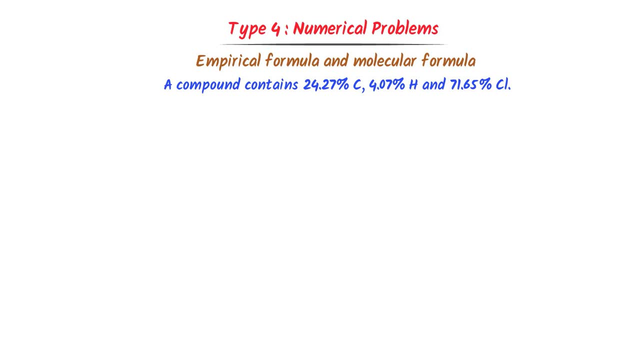 the carbon inside. the molecular formula is still 2.. cuatro por ciento carbono Here, 1.65% chlorine. Its molar mass is 98.96 g. Find its empirical formula and molecular formula In such type of numerical problems. firstly I find the empirical formula and then I find 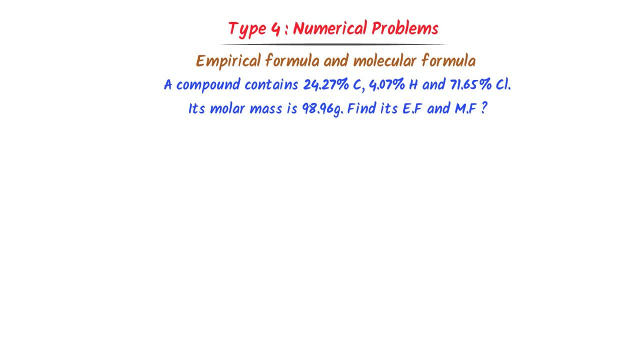 the molecular formula. To find the empirical formula, I will follow the three steps. In the first step I write the given atoms, like carbon, hydrogen and chlorine. Secondly, I write their respective atomic masses, like 12 g and 35.5 g. In the second step, I find: 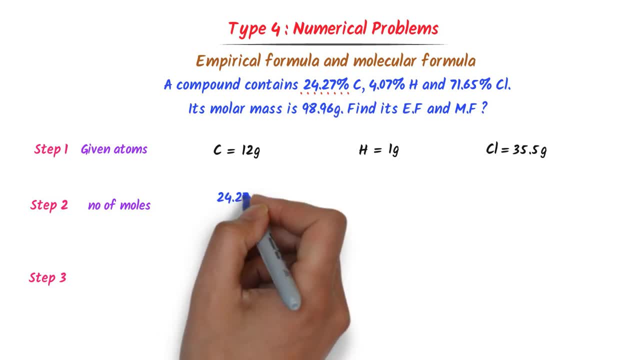 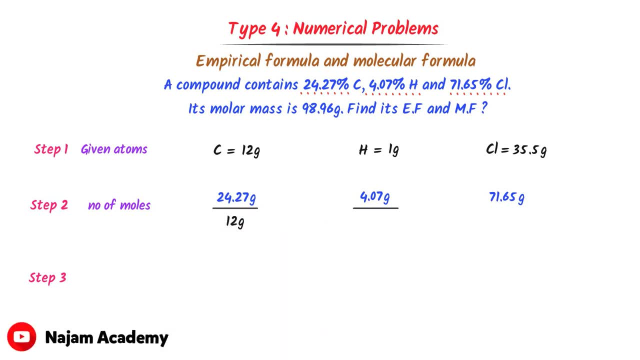 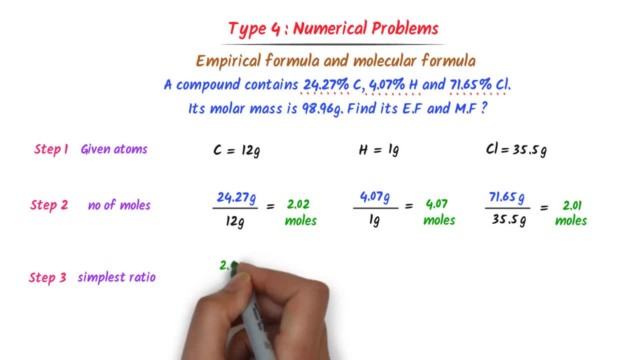 In the third step I find the simplest ratio. I rewrite these number of moles. The smallest number is 2.01.. I divide all these numbers by 2.01.. After calculation I get 1,, 2,, 1.. 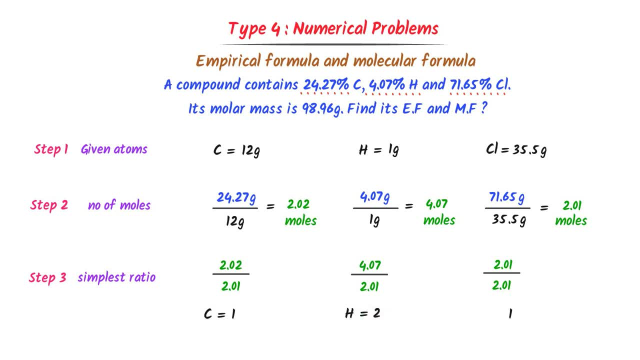 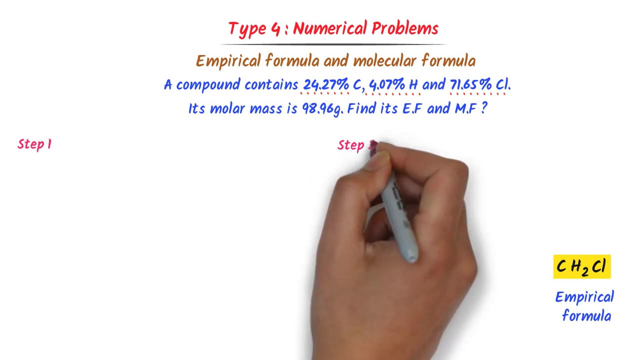 Hence the ratio of carbon is 1, hydrogen is 2 and chlorine is 1.. Thus, the empirical formula of the compound is CH2Cl. Now what about its molecular formula? Well, to calculate it, we have to follow two steps. 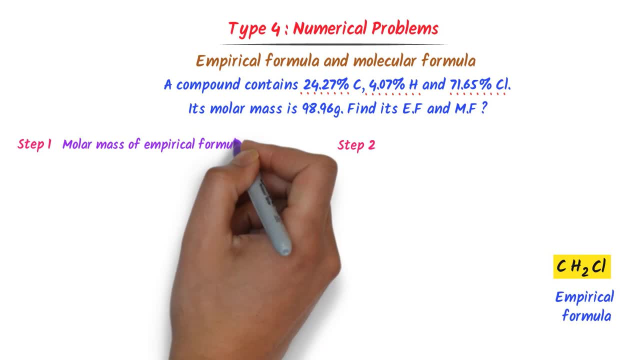 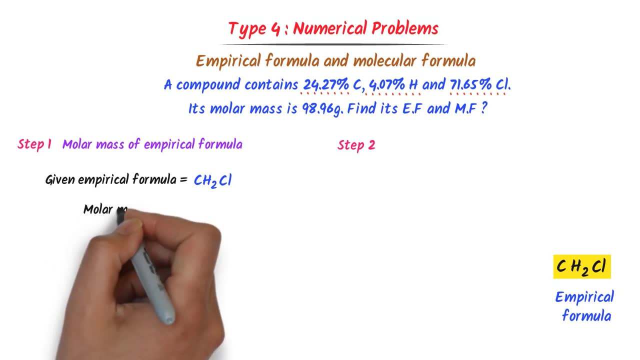 In the first step I will calculate molar mass of empirical formula. We know that the empirical formula is CH2Cl. I write carbon plus two hydrogen atoms plus chlorine. The atomic mass of carbon is 12 gram, that of hydrogen is 1 gram and that of chlorine is